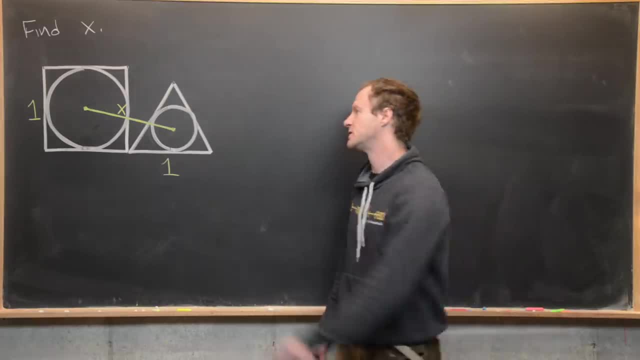 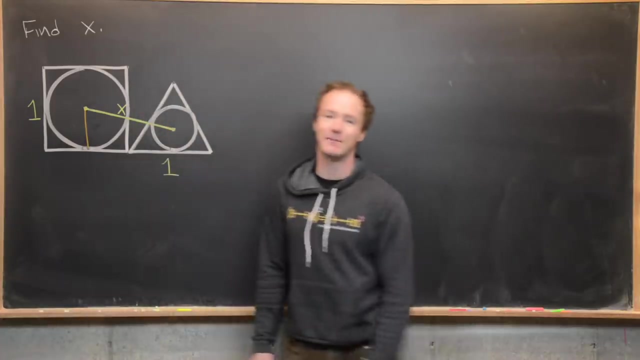 find the radius of each of the circles, So this radius of the circle inside the square. that's not too hard to see. So notice that we can just drop a line vertically from the center of this circle down to this side right here and it's going to bisect. 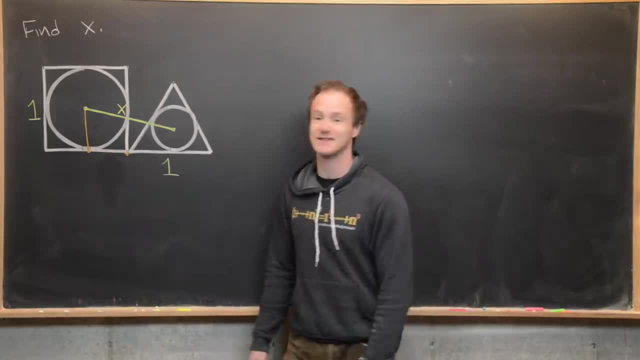 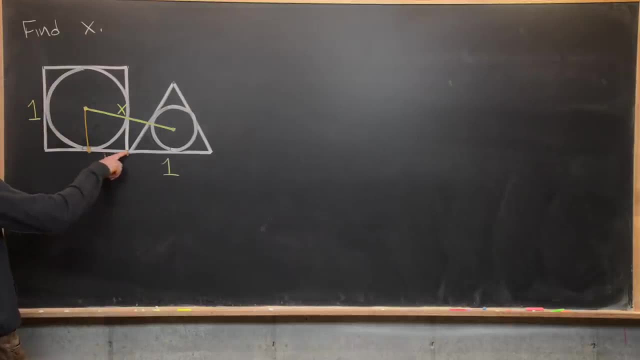 this side length. So now the fact that it bisects this side down here means that we have a length of one half, and that's going to be between this intersection point right here and then this corner of the square. But then, by symmetry, that also means that this length right here would be one. 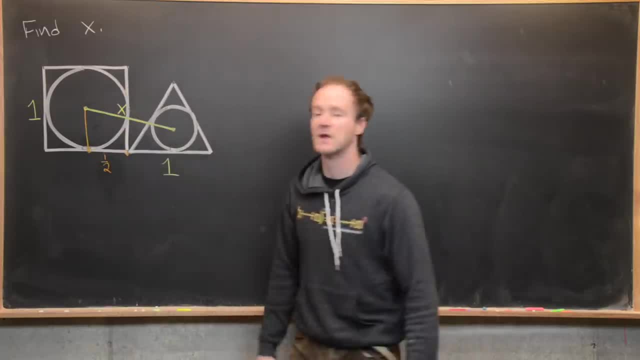 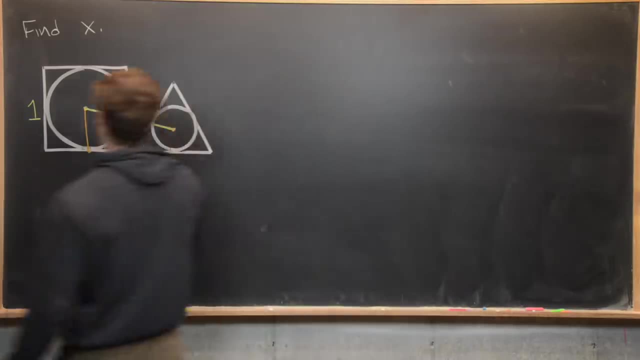 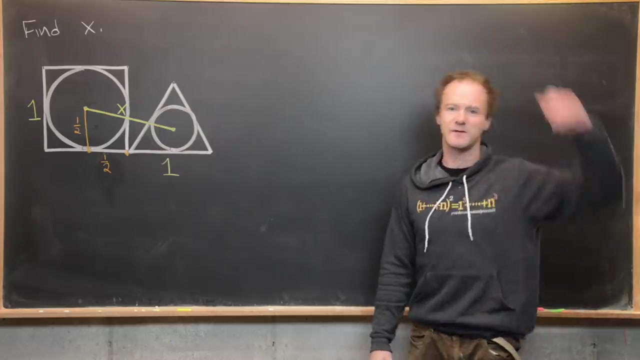 half if we were to make a horizontal line across. But then we've just created a sub square in here that all has length one half. But that sub square, one of its sides is a radii of the circle. So that means this circle has radius one half. 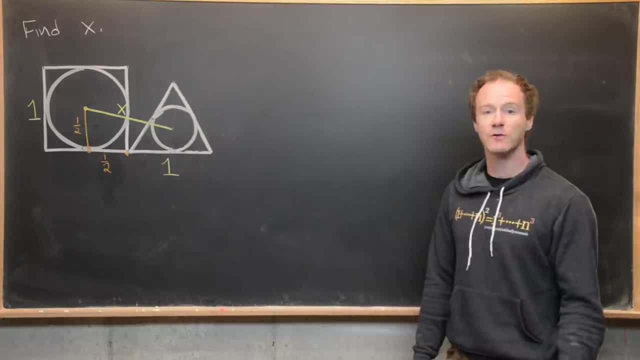 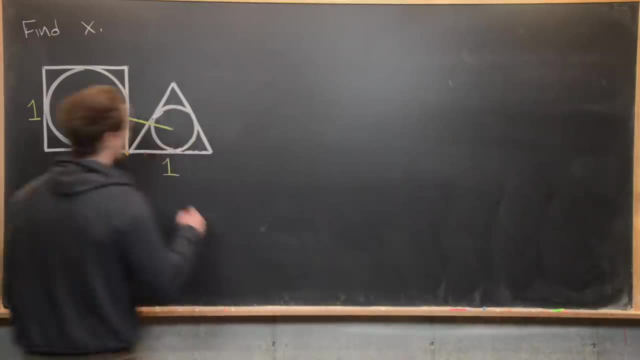 So that was super easy, Barely an inconvenience. Now we're ready to find the radius of the circle which is inscribed inside of our equilateral triangle. So I'm going to start by making a line segment from the center of this circle down to this intersection point right here. 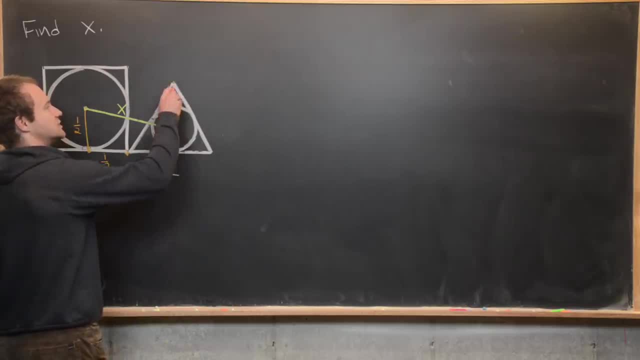 And then I'll also extend this line segment up to the top vertex of the triangle at such Great, And maybe the first thing that we want to do is calculate this distance right here. And actually this isn't too bad because we know this angle right here, So that's a right angle. 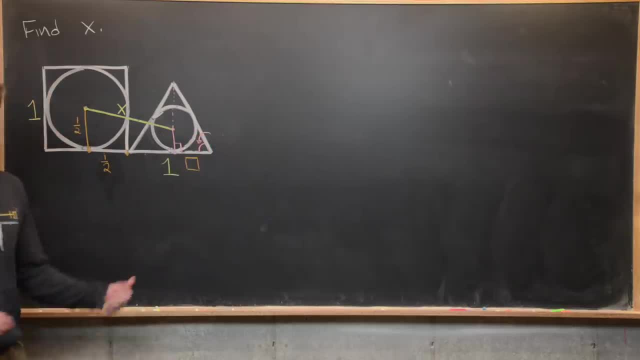 And then we know this angle right here. So that has measure 60 degrees again, because it's an equilateral triangle, which is pi over three radians. But now we can use some trigonometry, In fact we can use the cosine function. So we know that cosine of pi over three is going to be equal to whatever this. 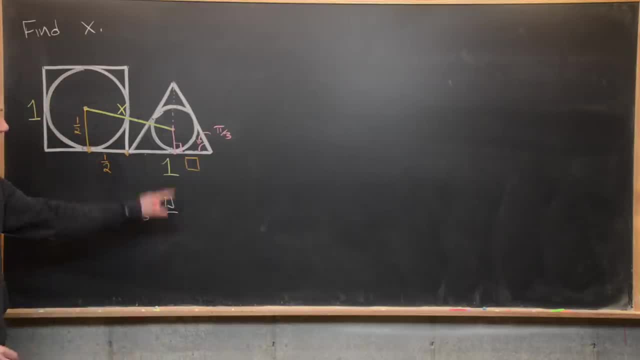 length here is, which I'll just put by a box over the hypotenuse. But the hypotenuse is the side length of this equilateral triangle which is just equal to one. But then on the other hand we know that cosine of pi over three is half. So that tells us that this length right here is one half. 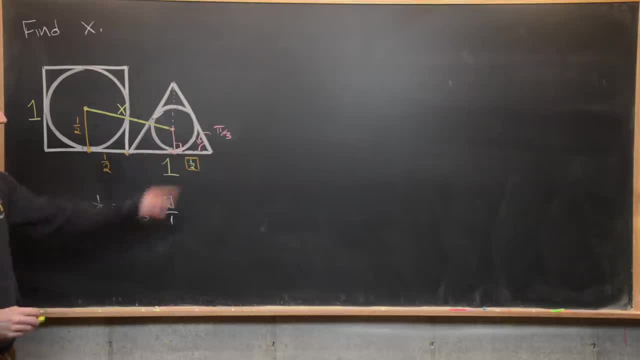 In other words this pink line segment, by sets our side length of our equilateral triangle. So we've got a side length of a half or half side length over here as well. OK, So that's actually good news, because we can use that to calculate. 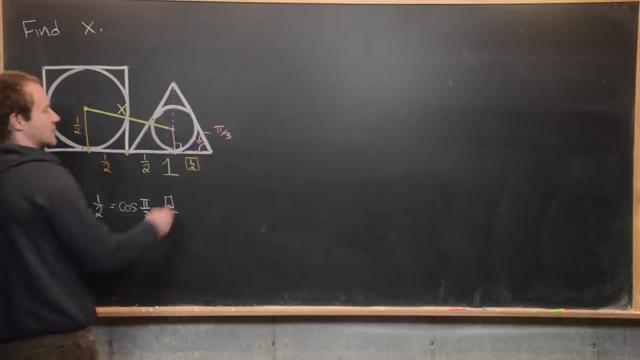 this radius of our circle. We can do that in the following way: So now I'm going to go ahead and draw a line segment from here to here and then, by a symmetric argument to what we've just done, we can use that. So this is going to be length half and this is going to be length half. 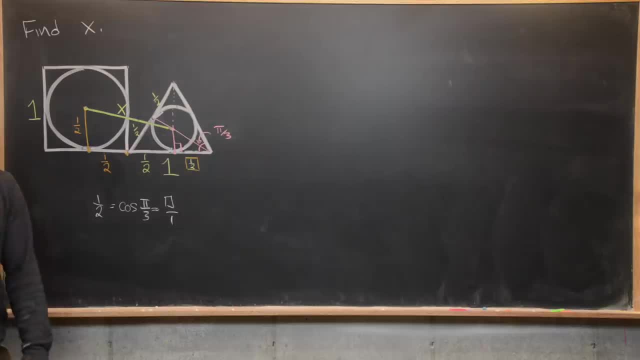 Which tells us that we have broken our equilateral triangle into two similar triangles by the side side side theorem. So notice, it's going to be this triangle right here and this triangle right here, So they share this pink side length and then all the other measurements are the same. So we've got. 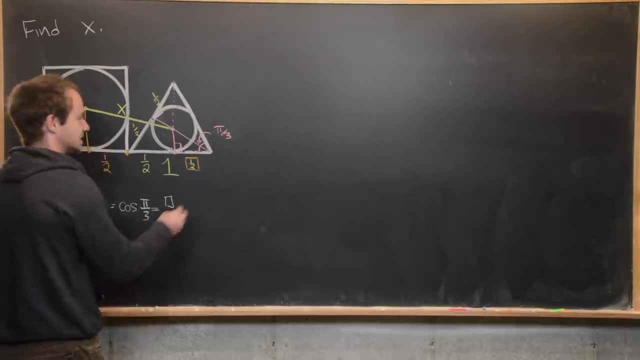 side, side, side equivalence there. But what that tells us is that this angle is actually being bisected. So that means we know half of this angle is pi over six. Now maybe we'll name this radius r and we can use again some trigonometry to calculate r. So notice, in this case we're going to 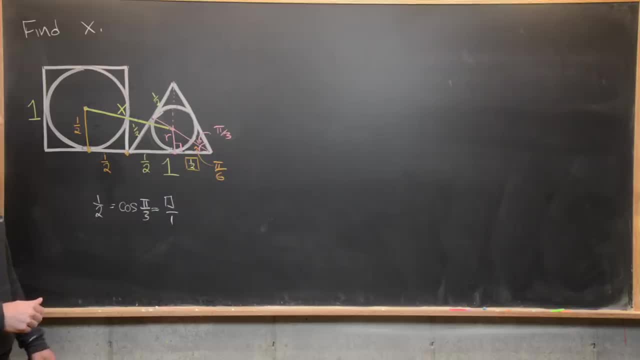 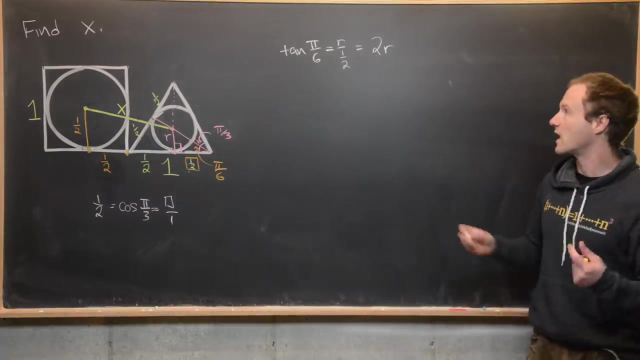 use the tangent function. So we know that the tangent of pi over six is going to be opposite over adjacent. So that tells us that tangent pi over six in this case is going to be opposite, which is r, over adjacent, which is half. In other words it's going to be equal to 2r, But then on the other, 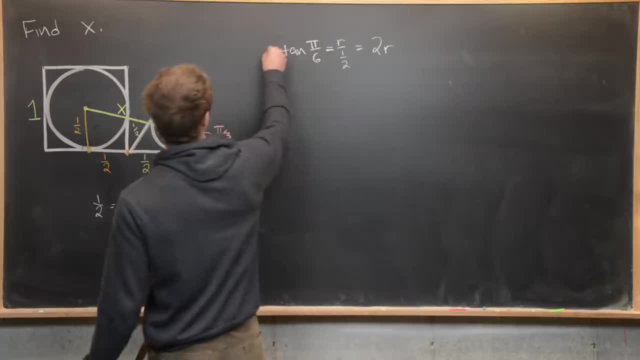 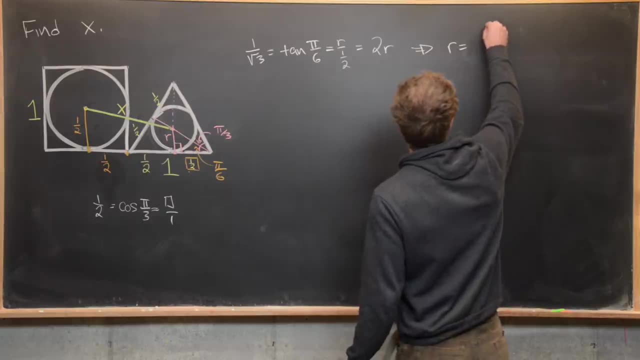 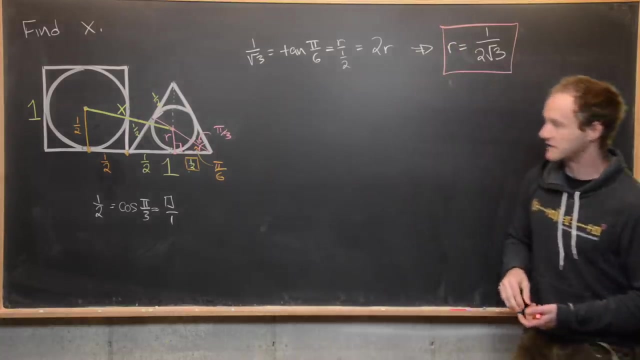 hand. tangent of pi over six is a well-known value. that's going to be one over the square root of three, so that tells us that our radius will be equal to 1 over 2 times the square root of 3.. So that's good news. We've got the radius of the circle that is inscribed in our equilateral. 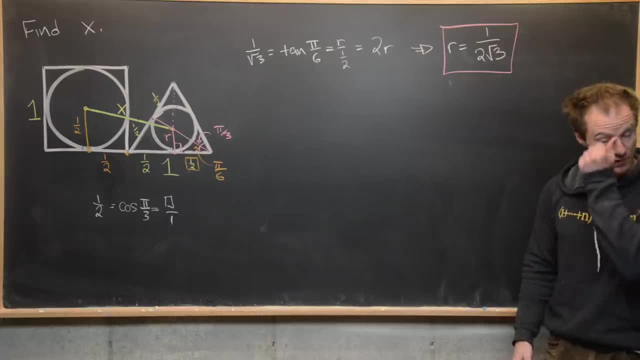 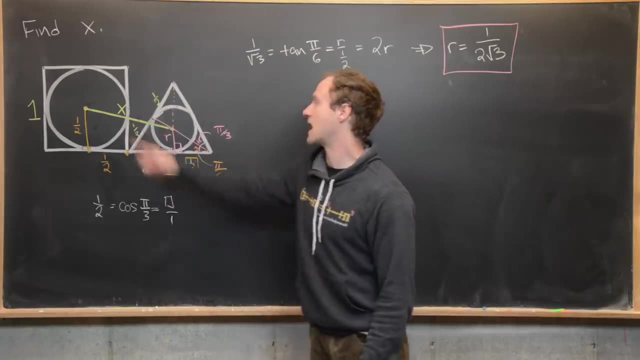 triangle WhatsApp, And now we're actually in good shape to finish this problem off. So what I'll do now is create a triangle. well, it's gonna be a right triangle whose hypotenuse is this: goal, value x. So let's go ahead and do that. 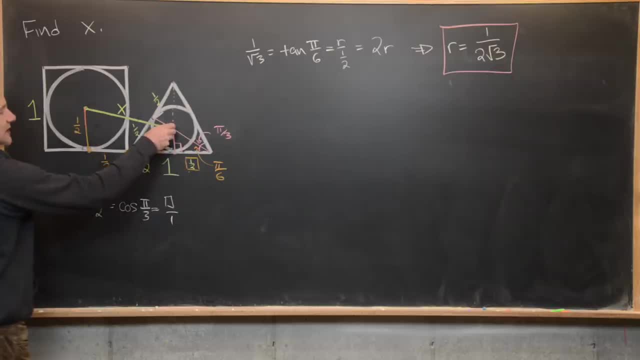 So it's gonna look something like this. So I'll make a line parallel to this side of our square and our triangle, but it is going to go from the center of this circle. Good, And then we can easily measure the two lengths of the sides of this right triangle. 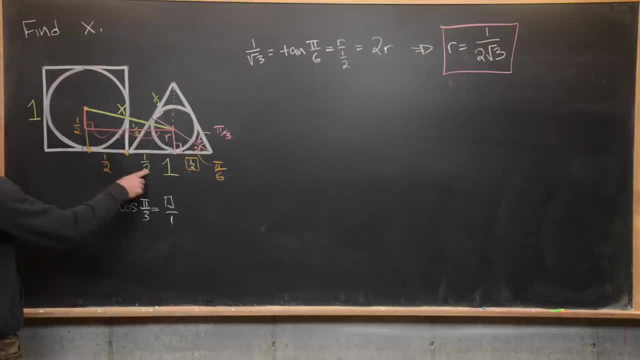 So notice that this length right here is gonna be 1 1⁄2 plus 1 1⁄2, so this length is one. And then this length right here isn't too bad to calculate either: It's gonna be 1 1⁄2,. 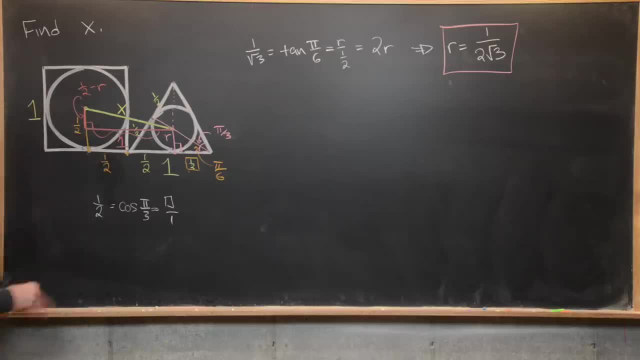 that's gonna be this entire distance here, minus r. that's because this is just the transposed radius of this inscribed circle over here. so 1 1⁄2 minus r. But we know what r is. r is gonna be 1 over two times the square root of three. 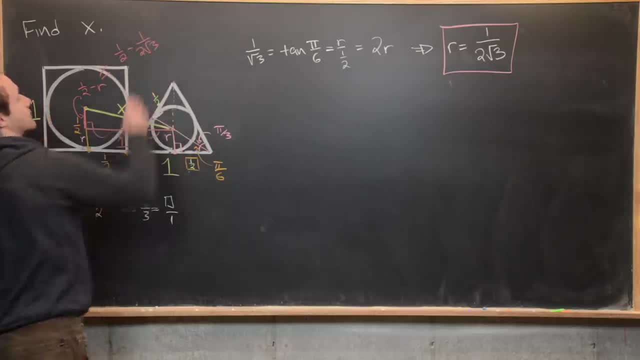 so this is 1 1⁄2 minus 1 over two root three. But now, finding a common denominator, we pretty easily see that that's gonna be root three minus one over two root three. So let's see what we've got here. 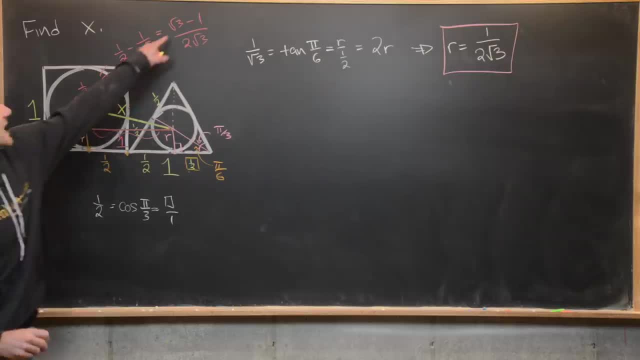 We've got a right triangle, side length one, and this object and hypotenuse x And we're gonna use the Pythagorean Theorem to calculate our x. So let's see what we have here. We have: x equals the square root. 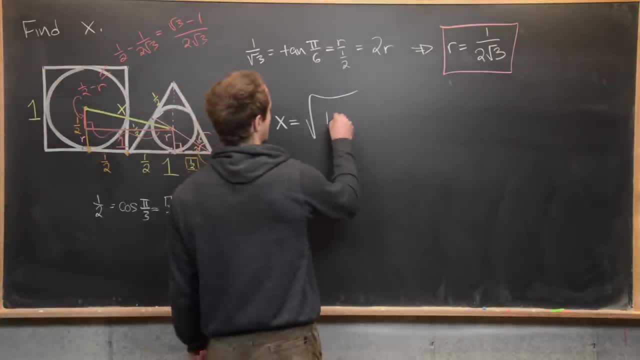 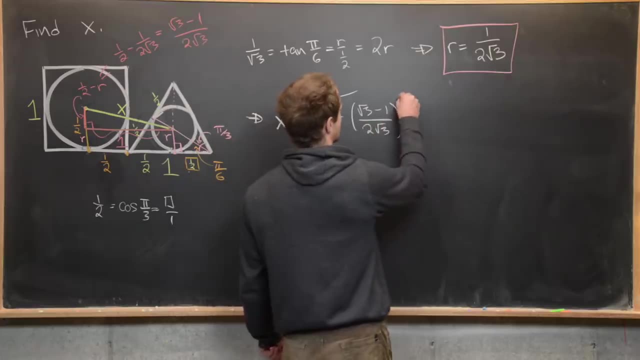 of the sum of the squares of these two things. So it's gonna be one squared plus, and then we'll have root three minus one over two. root three, quantity squared. So we have something like that. So now let's go ahead and calculate this. 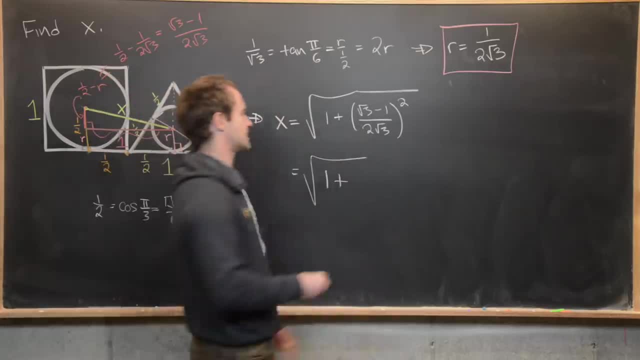 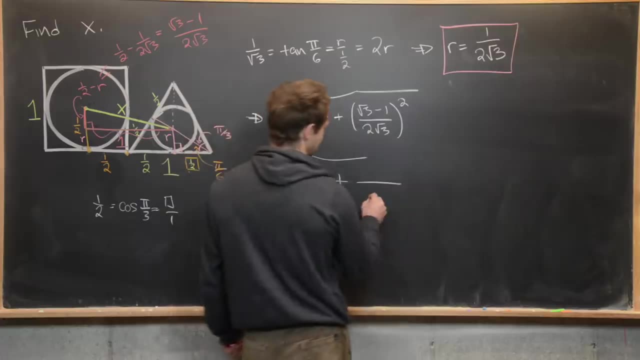 So that's gonna give us the square root of one plus. So notice our denominator here is pretty easy to write down. We have two squared, which is four times root, three squared, which is three, So that's gonna be four times three, which is 12.. 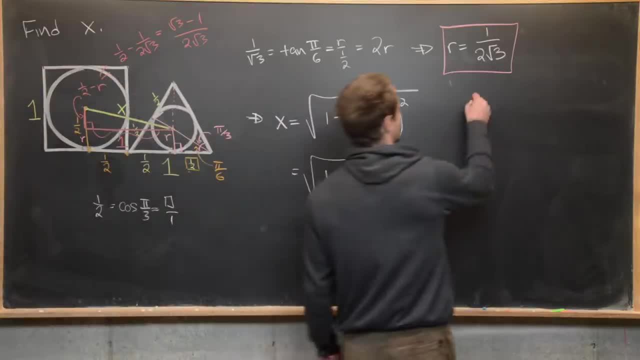 And then our numerator. we can just FOIL that out, So maybe we'll do that over here. So we've got root three minus one times root three minus one. So that's gonna give us root three times root three. That's just three. 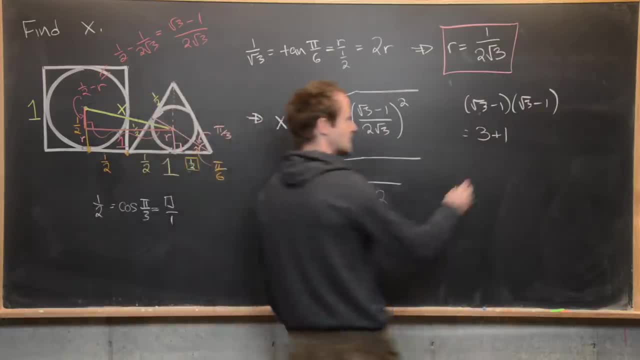 Negative one times negative one, so that's plus one. And then notice we're gonna have minus two root three from the cross terms. So that's what we get from this side calculation of squaring out that term. Good, so let's maybe go ahead and write that over here.